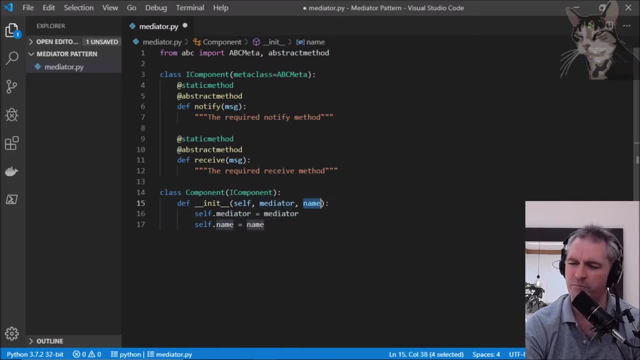 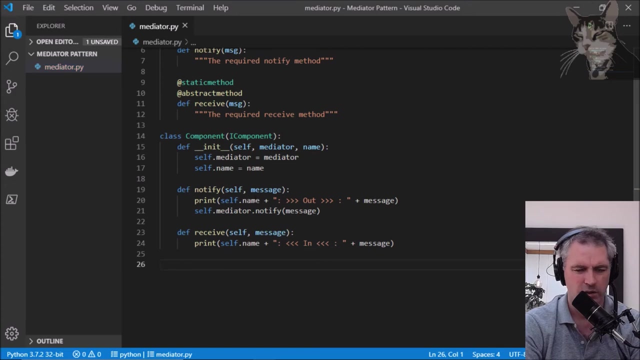 and we can also tell the component its name. Okay, so now I'm going to add a required notify method to components. so define notify, mediatornotifyMessage and I'll add the receive method. Okay, excellent, Now let's create the mediator. so class mediate or. 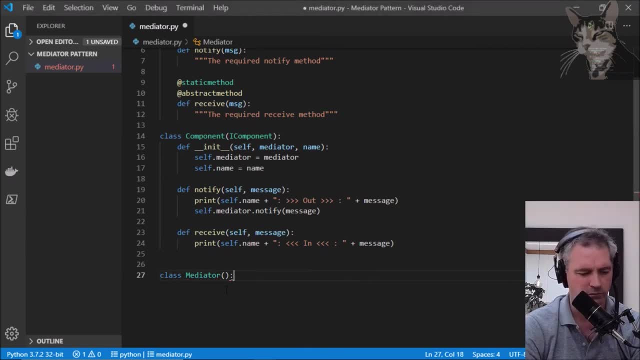 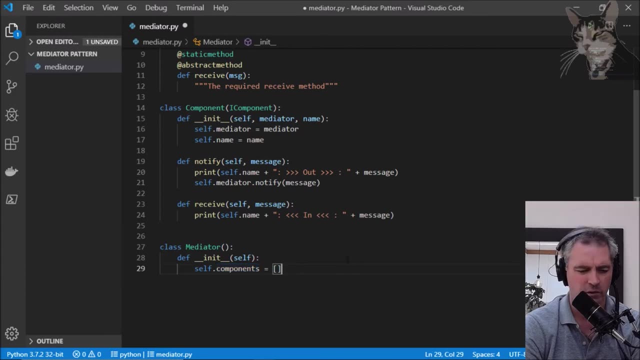 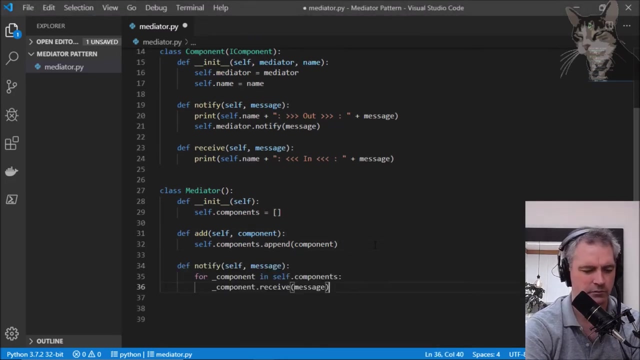 it has an init function And it keeps a list of components that it knows about. We'll create an add method so that we can add components and we'll add a notify method so that we can notify all components. Okay, so, for all the components and self components, we'll call the components receive method- receive and we'll call the receive method. 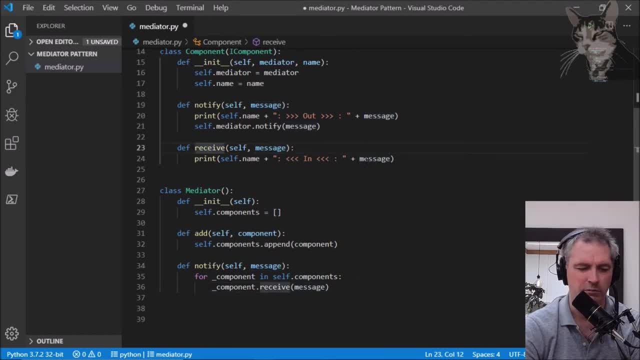 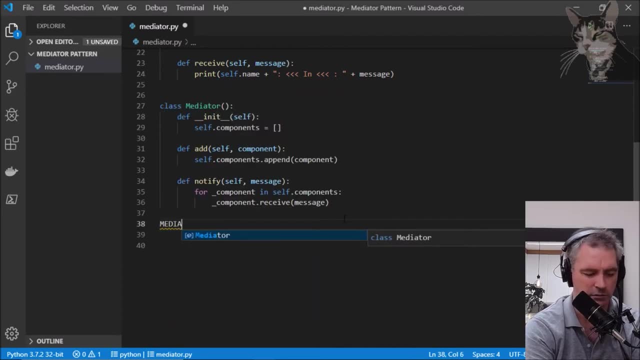 receive and we'll print out the incoming message. okay, so let's create now a client called me ta tour. we call same mediator and we'll create a component. one equals a component and it needs no better mediator. so there's a mediator and the name of the component is component one. let's 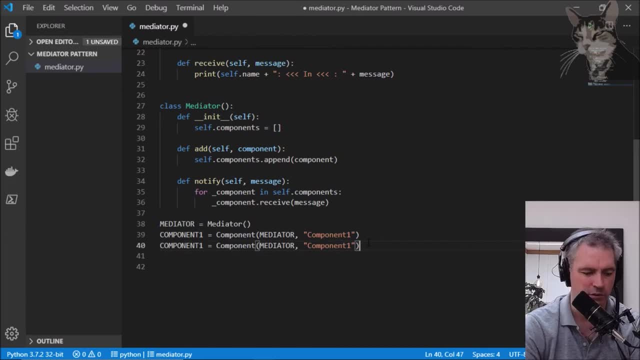 create another component called component two and another one called component three. we have three components. now we'll also add those components to the mediator. so mediator dot add- add component one, mediator dot add component two and mediator dot add component three. now we'll test this out by making component one. 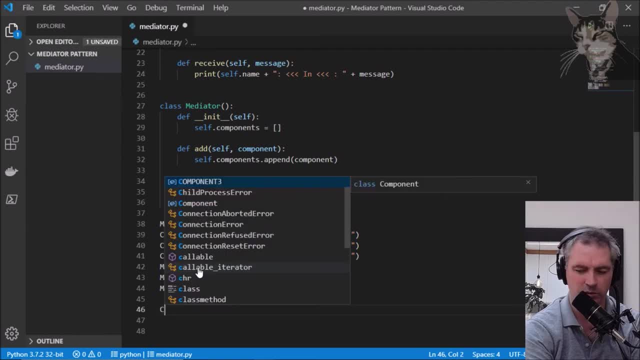 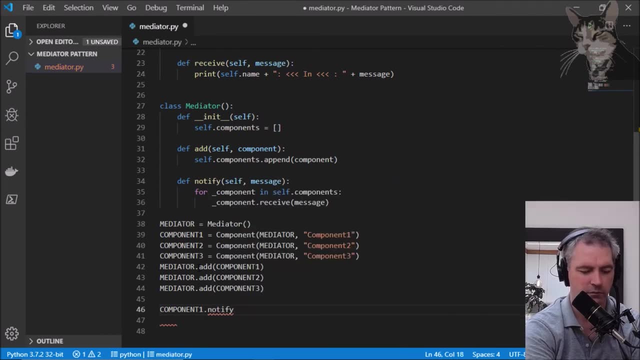 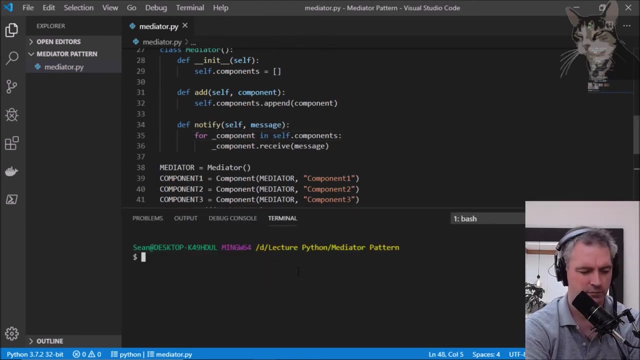 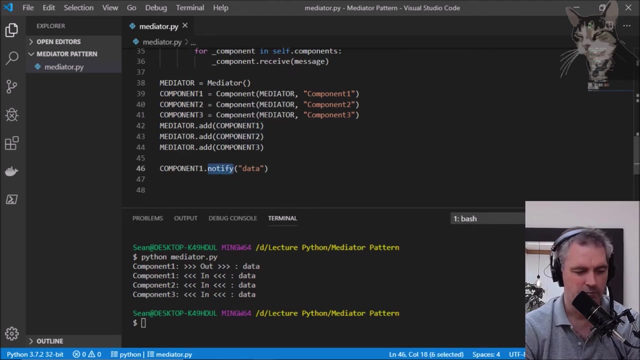 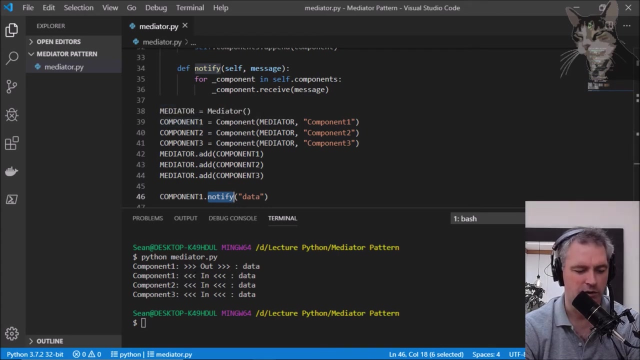 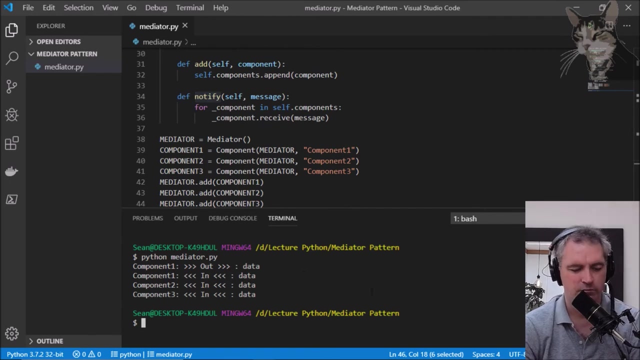 send a message to all other components. so component one dot notify everybody of data. okay, let's try that out. python mediator dot py. okay, so component one sends data using a notify method and the mediator, which has a list of all components, will then each component's receive method and in comes the data in. so we can also do component two dot notify. 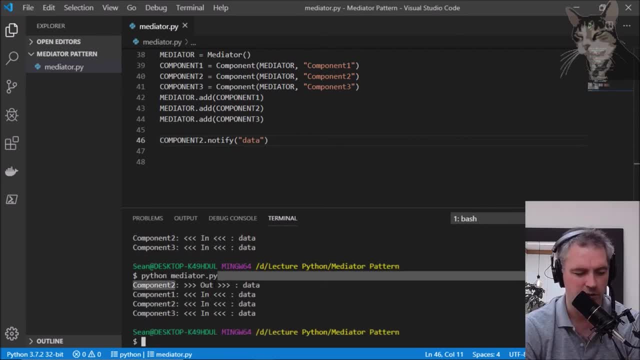 and see the way around. well, component two goes out and the mediator sends data back to each component. now the great thing about the mediator is that we can tell it to not send data back to the component sending the data. we'll just extend this slightly. going up to the component, 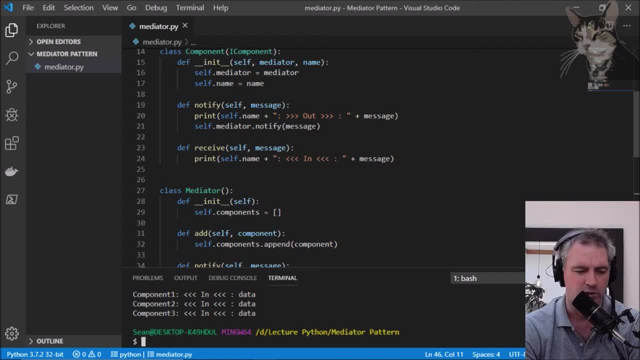 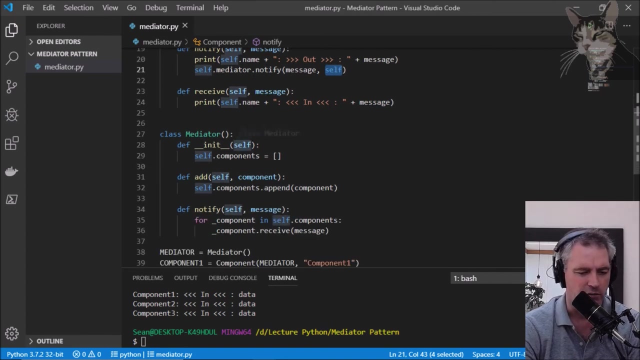 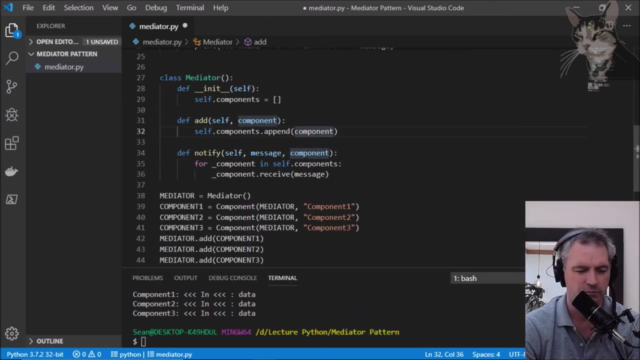 when the component notifies, it also tells the mediator who it is by using self. okay, so, mediator, notify the message, but we'll also pass a reference to ourself. so in the mediators notify, we also need to know about which component was the sender and so if 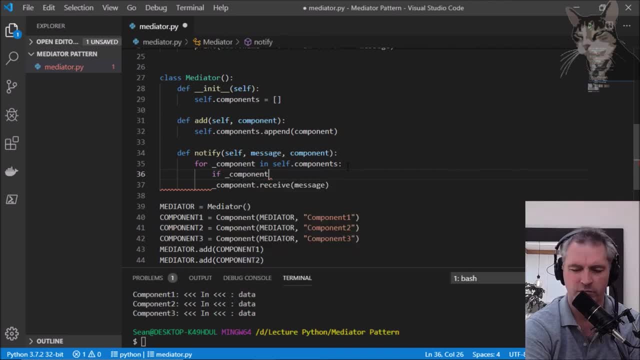 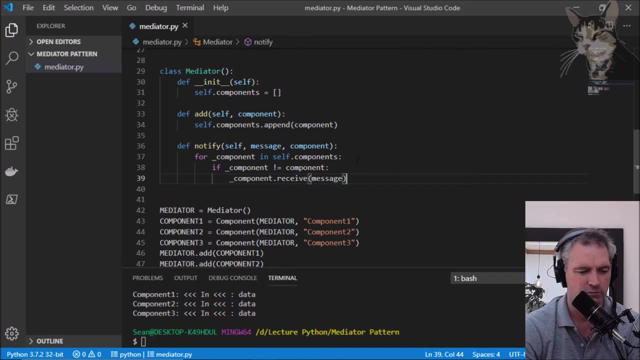 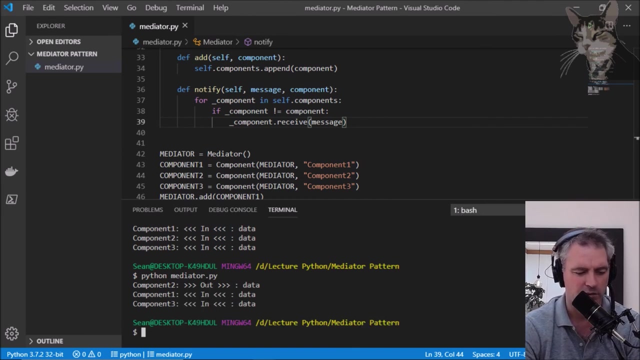 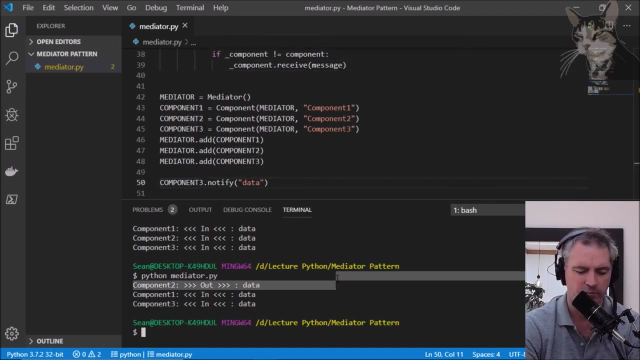 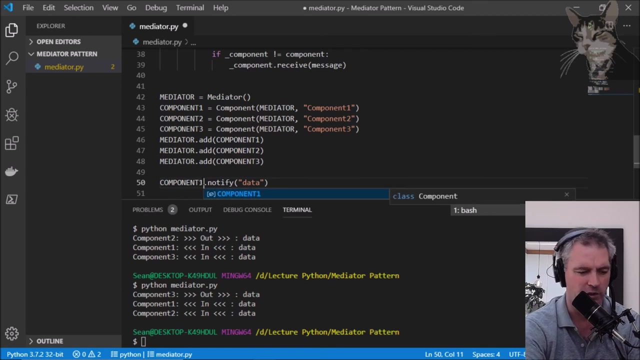 component is not equal to the component, then we can call all other components receive methods. let's try that out. okay, so component two out and only component one and three got incoming data. so let's try that with a different component three. three sent data out and only one and two got data in, and really that's. 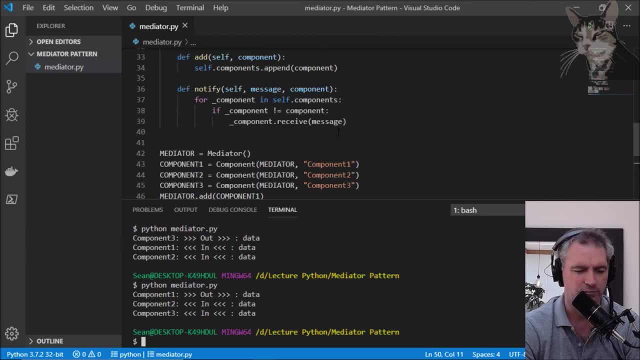 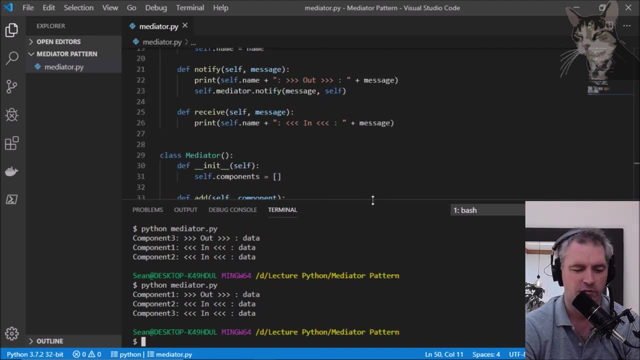